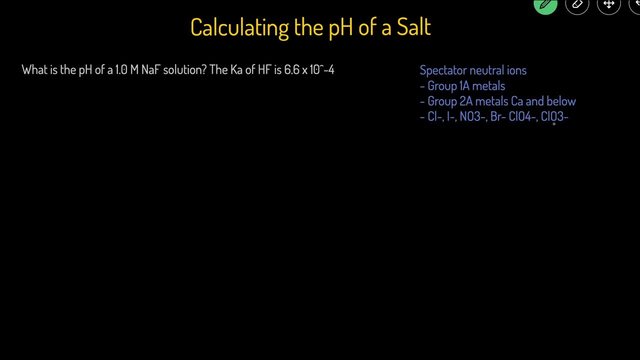 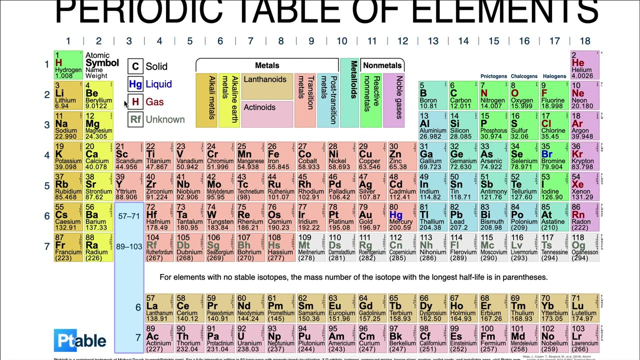 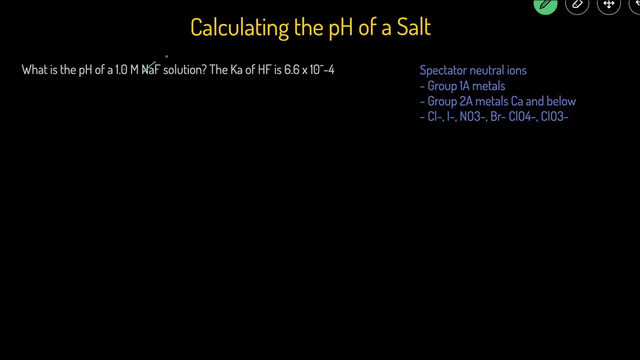 the group 2A, metals that are calcium below, and then these anions right here. So we will cross out the Na because Na is in group 1A. As you can see, right here Na is in the first group, So we'll cross out Na. and if we cross out Na then we'll be left with F minus because Na. 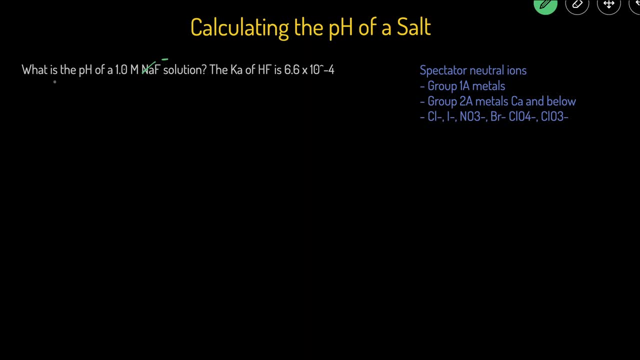 is a positive 1 charge, so F has to be a negative 1 charge. So really this is asking: what is the pH of a 1.0 molar F minus solution, F minus. since this has a negative charge, we know it's going to. 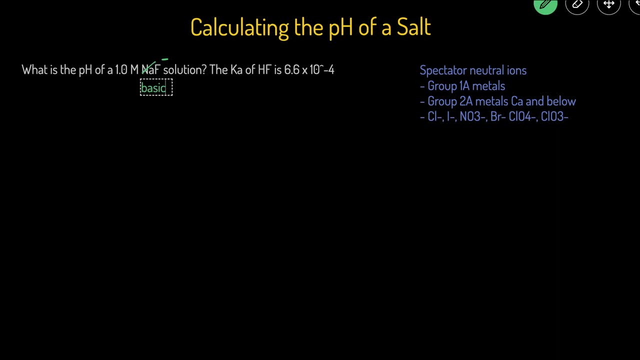 be basic. So this just comes down to calculating the pH of a weak base. We can use the Kb shortcut or we can use the full process. I'll show you the full process and I'll show you the Kb shortcut afterwards. So we can start by writing out the reaction: F minus plus. 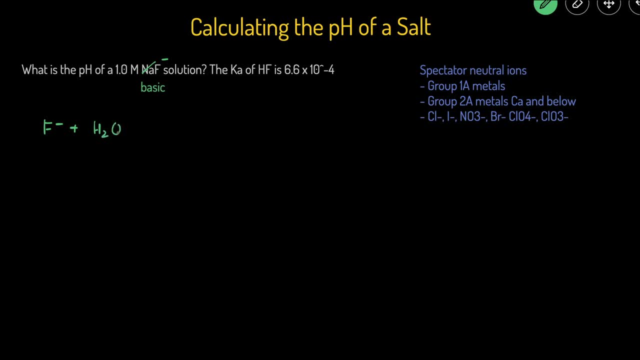 H2O, because this is the H2O in the solution. where water is the solvent, Then we'll get a reaction. F minus is the base, so it's going to accept a proton from the acid. H2O is acting as. 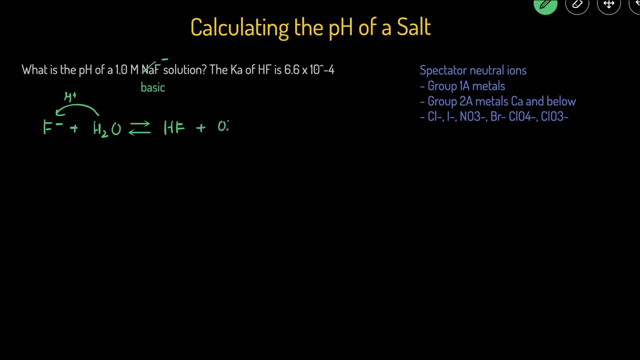 the acid here and we'll get HF and OH minus. I have a double-headed arrow here because this is a weak base. Then we can set up an ICE table. The initial concentration of the F minus was 1.0.. Water is a liquid, so we can just ignore it And the original concentration of HF and OH minus. 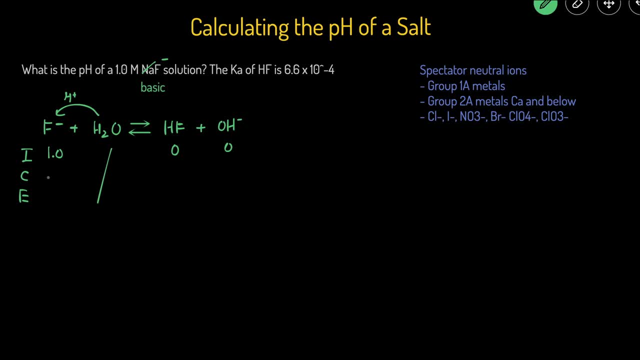 they're both zero, because this question doesn't mention anything about them. C will be- C stands for a change, F's C line will be minus X, and the HF and OH. they're both going to be plus X. And then E is just the sum of the I and C lines. This will just be 1.0 minus X. 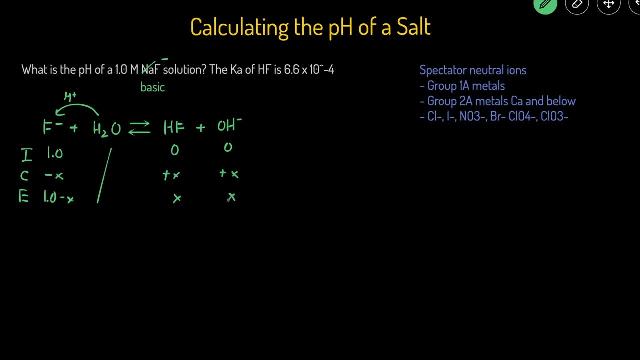 zero plus X is just X, and zero plus X is just X. Now that we have equilibrium values or the equilibrium variables, we can plug this into the Kb expression or we have to plug it into actually the Kb expression. So we're given the Ka here, but since F minus is a base, we have to use Kb, not Ka. 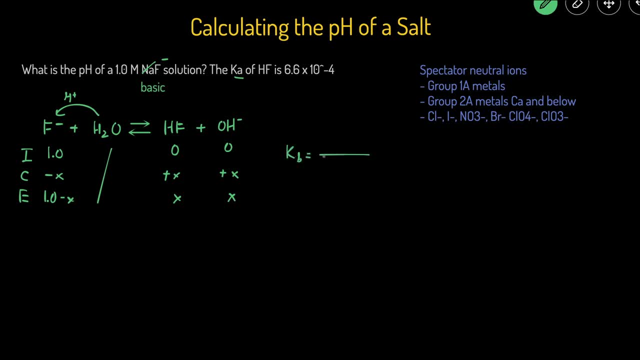 So let's just set up the Kb expression for now. The Kb expression is this: concentration of products divided by concentration of reactants. So this will be X times X, X squared on top, and then the bottom will be 1.0 minus X squared on top, And then the bottom will be 1.0 minus X squared on top. 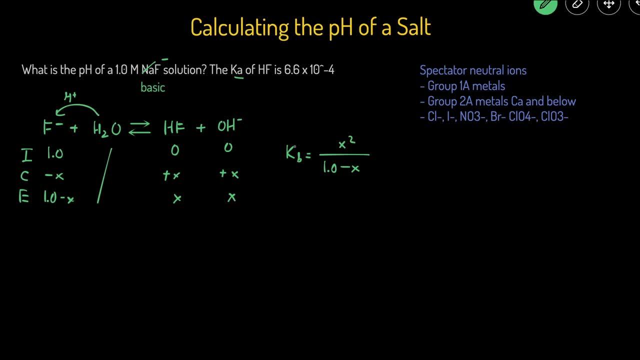 But we have the Ka, we don't have the Kb. So to calculate the Kb we can use this equation: Ka times Kb equals 1.0 times 10 to the negative negative 14.. Then Kb is just going to equal 1.0 times 10 to the negative 14 divided by the Ka, which is 6.6 times 10 to the negative 4.. 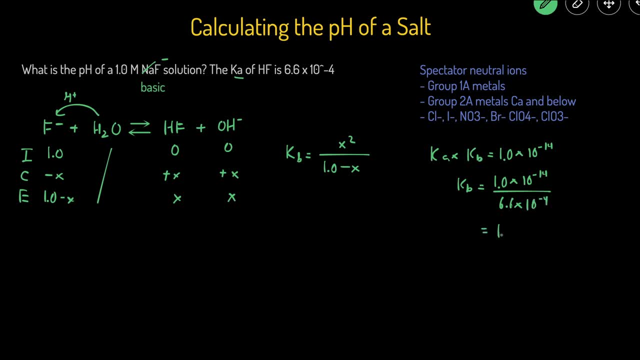 We're given that value, That comes out to be 1.51 times 10 to the negative 11.. So that's our Kb. Let's plug it in right here. That's going to equal X squared divided by 1.0. 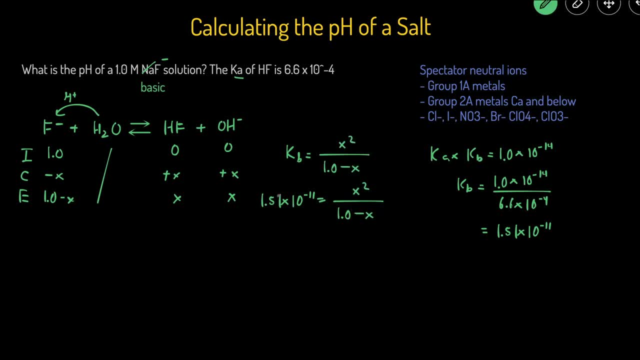 minus X. But since Kb is so small, it means this reaction doesn't really happen much. So that means the X is going to be extremely small and we can ignore the minus X Pretty much if the K value is to the negative four power or less. 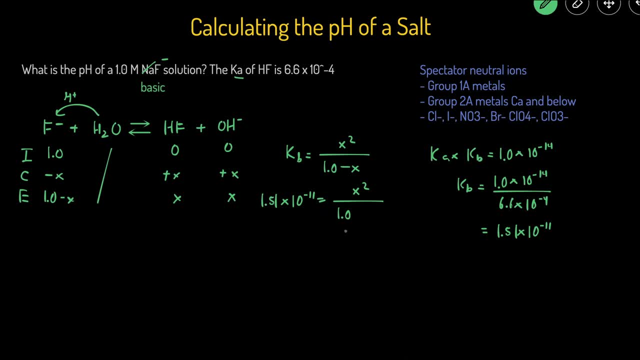 like negative five, negative six, then you can just ignore the minus x, then we can just multiply both sides by one and then take the square root of both sides to solve for x. so it really just comes down to square rooting this number right here, and so x is going to equal 3.89 times 10 to the negative 6. 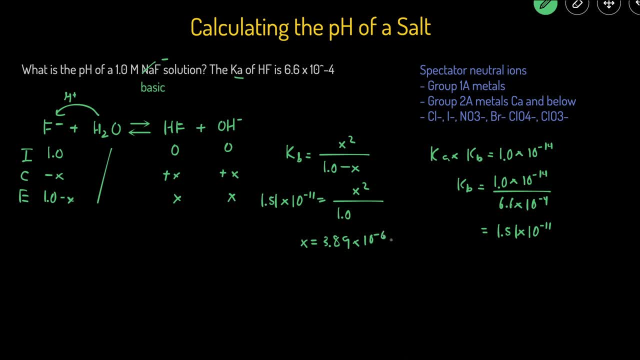 and x is equal to the concentration of hydroxide, so that's the concentration of the oh. now we have oh, we can figure out the poh, which is going to equal negative log of 3.89 times 10 to negative 6, that's 5.41. and then, lastly, ph is just 14 minus poh, so 14 minus 5.41. 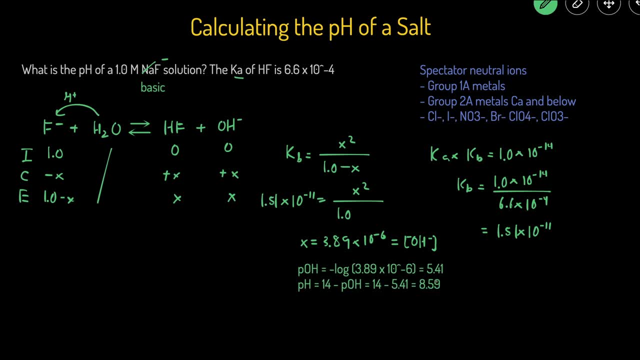 and that is 8.59. so, as predicted, the solution is indeed basic. the ph is above 7.. this is the full process for solving for the for the ph. once you know that the solution is basic, the shortcut, as i was mentioning earlier, is just the kb shortcut. you can go straight to. 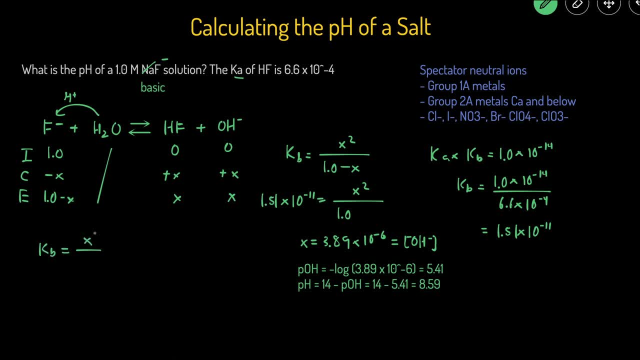 setting up kb equals x squared divided by the concentration of the base, instead of having to set up the ice table, so we can just skip the ice table and it comes straight to this. and then, if you, if you need more practice of this, just check out my my kb video where, or my video where i 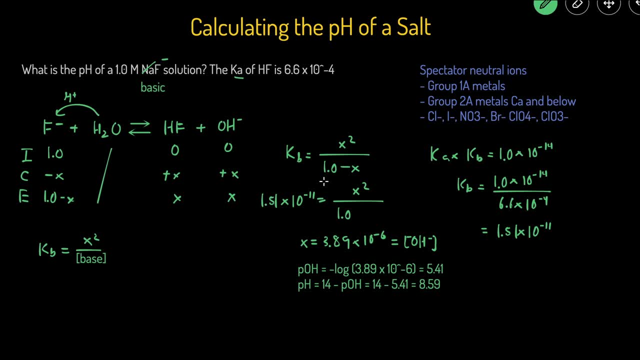 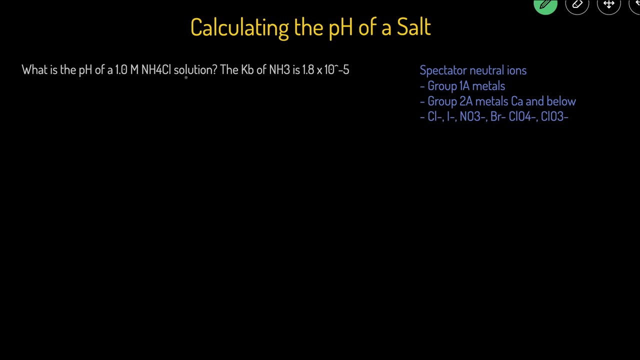 talk about how to calculate the ph of a weak base. let's try another problem, where we calculate the ph of a salt solution. this question reads: what is the ph of 1.0 molar ammonium chloride solution? we're also given that the kb of ammonia is 1.8 times 10 to the negative 5.. so the first thing. 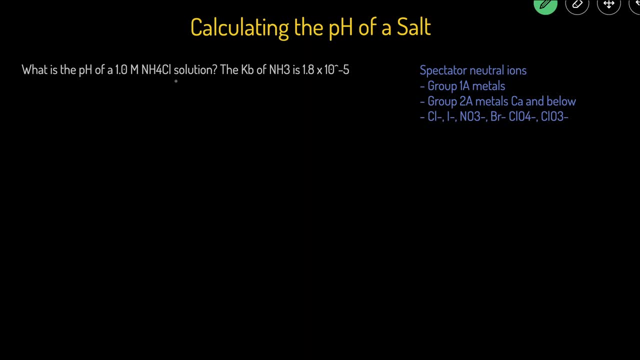 we should do just like in the last. problem is just get rid of any of the neutral spectator ions, which co minus is one of them. you can see right here. so we get rid of co minus, we're left with nh4 plus, and since this ion has a positive charge, it means it is going to be acidic. so we're just going. 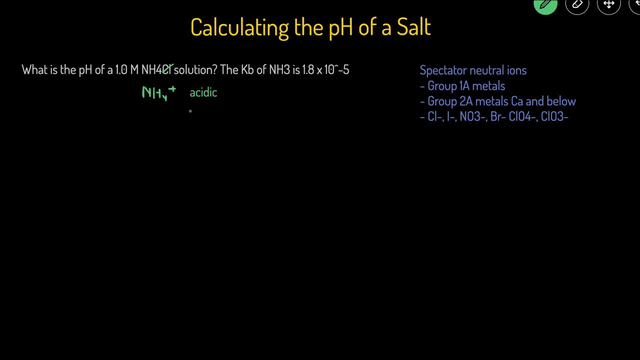 to be calculating the ph of a weak acid solution. we can write out the reactions of the ice table or we can just go straight into the ka shortcut. so since, again, this is an acidic solution, we're going to be using ka shortcut instead of kb shortcut. so ka shortcut. ka is equal to x squared divided by the. 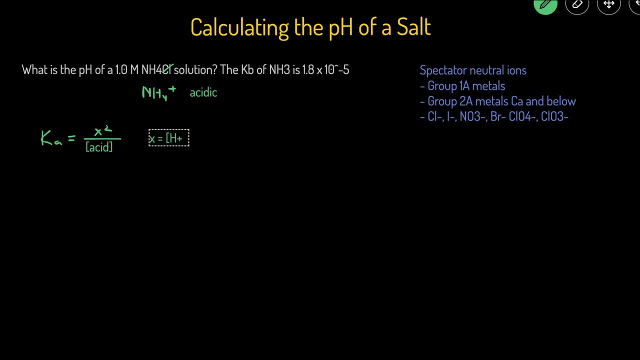 concentration of the acid. and once we get x, x is going to equal to h plus concentration and ph is just going to equal negative log of x. we have to kb. let's solve for the ka. well, k a is going to equal one times 10 to the negative 14 divided by dkb, which is 1.8 times 10 to the 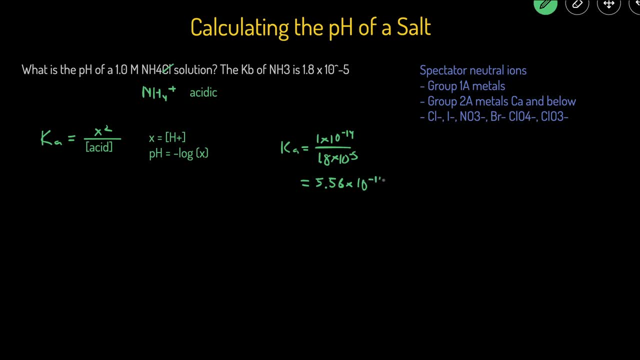 negative 5. that equals 5.56 times 10 to the negative 5. negative 10. so we'll put this right here: ka is equal to x squared divided by the original concentration of the acid, 1.0. and this is 1.0 because this is going to break up into nh4 plus. 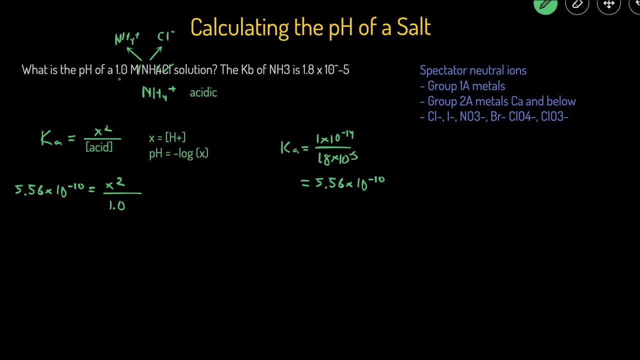 and cl minus and there's a one, one and one ratio. so if we start with one molar, we'll get one molar of both of them. then we can just multiple, multiply both sides by one and take the square root of that and we'll get our x value. x equals 2.36 times 10 to the negative 5 and x when you're using the.